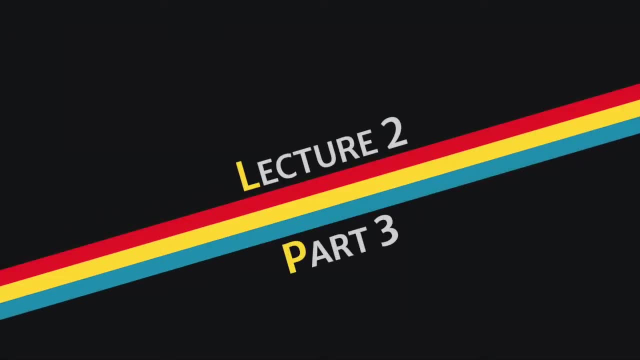 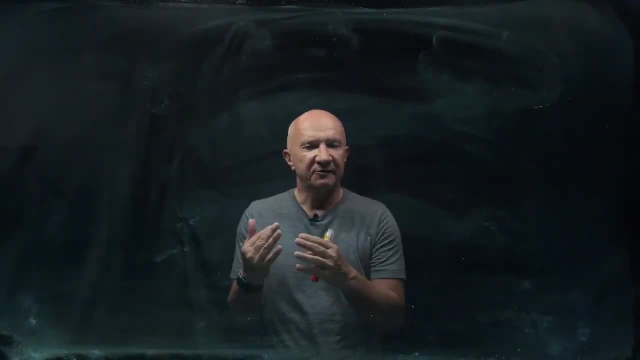 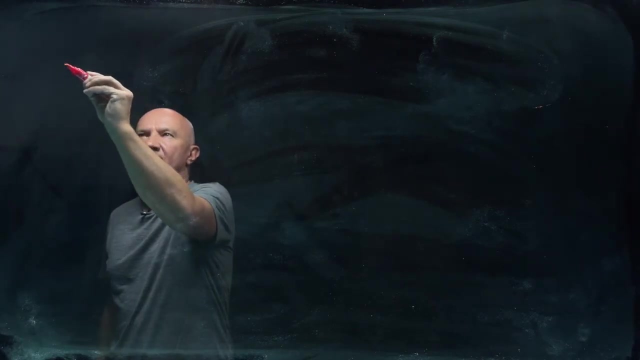 Probably the most important diagram for understanding quantum information science is that of single qubit interference. Let me draw the network for this. So I'm going to have a qubit that starts in state zero. It goes through the Hadamard gate, then followed by 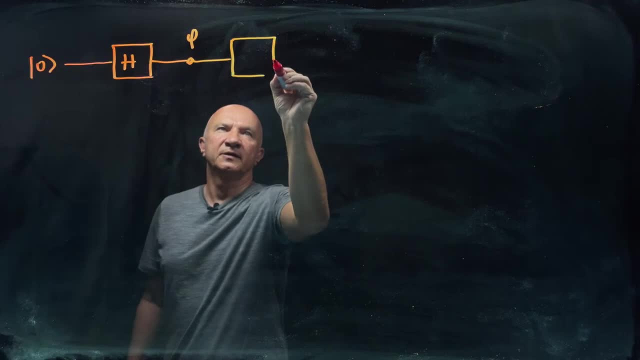 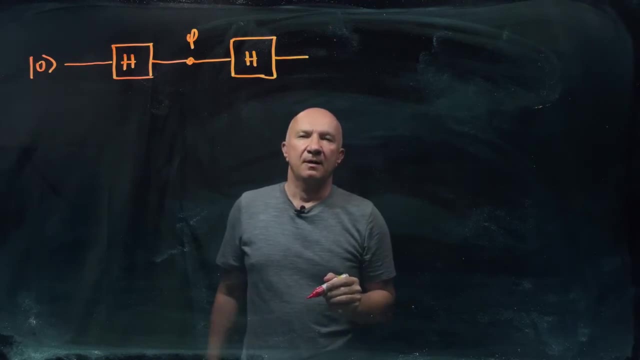 the phase gate and then followed by Hadamard gate, And then the qubit is measured at the output here And we want to know what are the probabilities that the qubit will be found in the ground state or the excited state. The elements of this diagram should be clear by now. 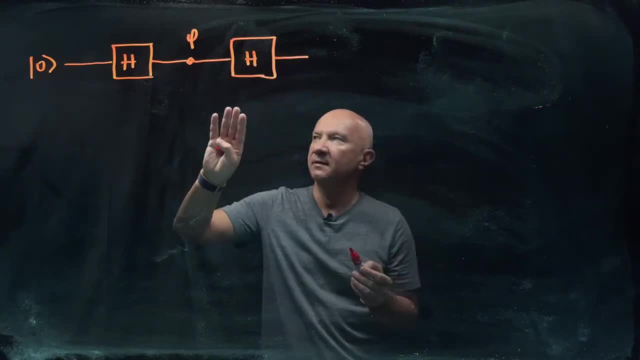 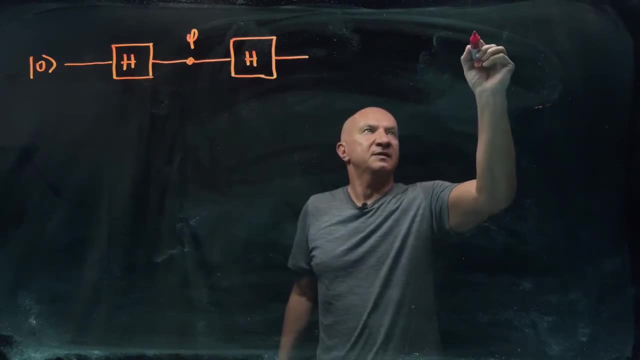 The horizontal line is my qubit. The three gates that I that you can see here are the qubit and the phase gate, And then the qubit is measured at the output. here You can see, here is the Hadamard gate. So the Hadamard let's. for completeness, let me just 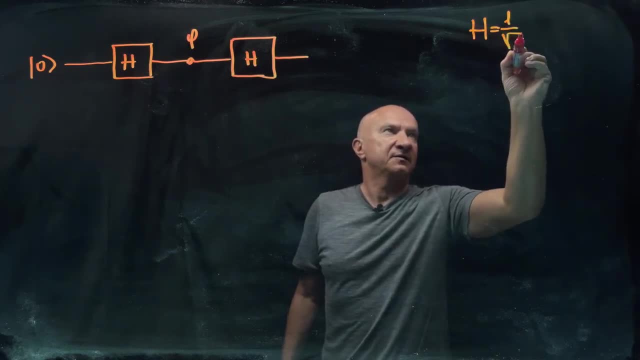 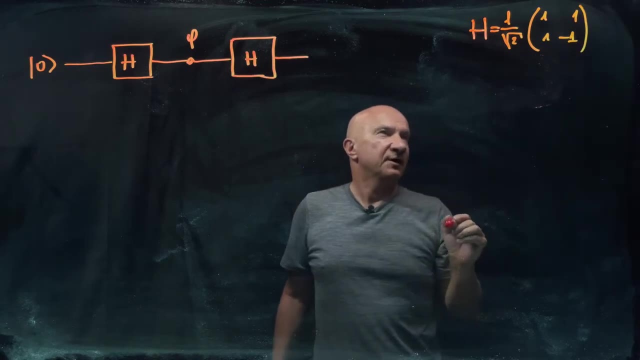 write the matrix corresponding to the Hadamard gate. So that's a unitary matrix that looks like this, And quite often, instead of writing it this way, we will characterize the Hadamard gate by the transitions. We'll write that zero goes to one over square root of two. 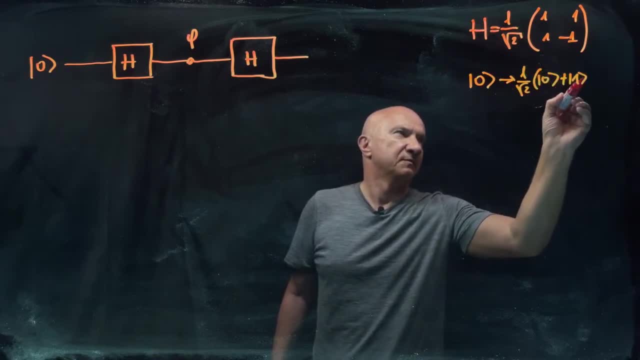 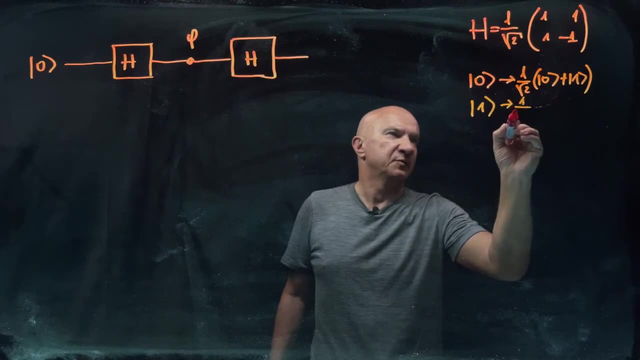 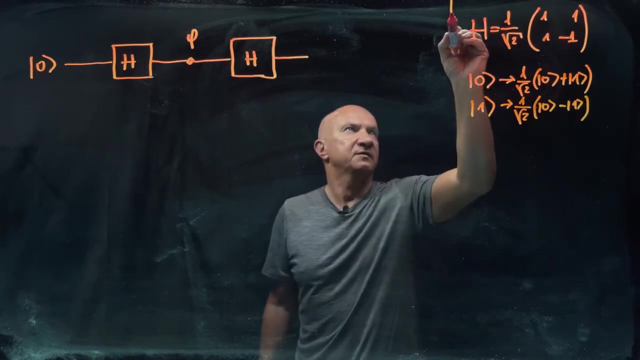 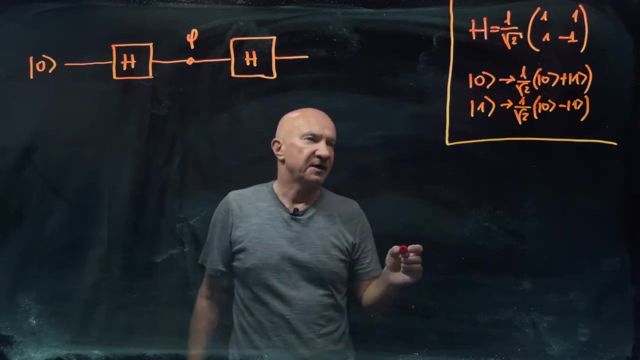 zero plus one And one under the Hadamard gate is transformed into a superposition, one over square root of two zero minus one. Okay, so this is actually one way of specifying the Hadamard gate. Then I have the phase gate here And the phase gate. I'll just write this: 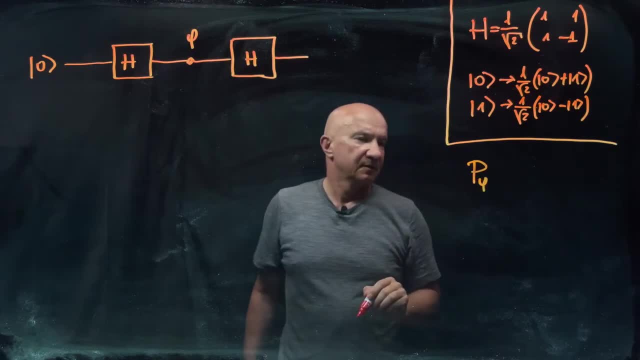 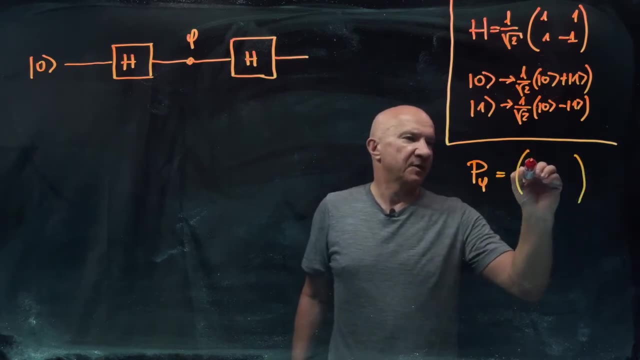 P and the phase shift will be here. So the phase shift is phi And the corresponding matrix is the diagonal matrix, with one here, EI phi, and zeros here. So that means that zero is transformed to zero, but one gets the phase shift, EI phi, one. So that's: 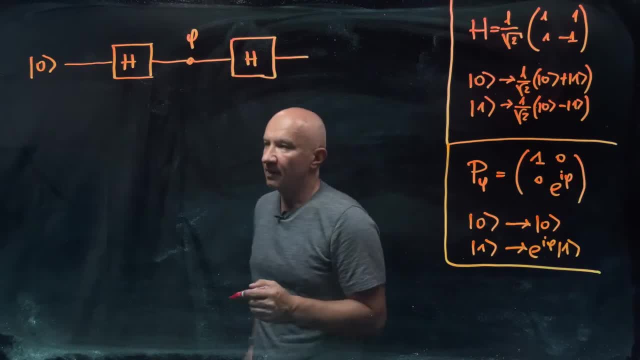 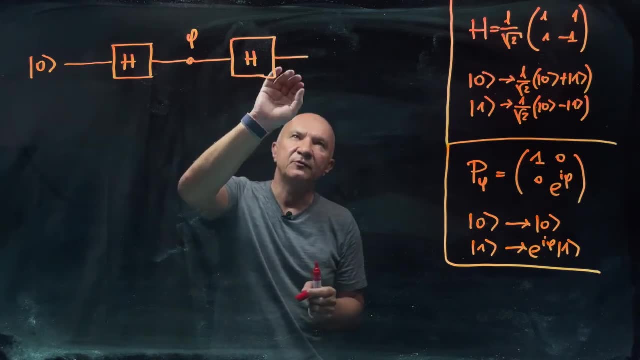 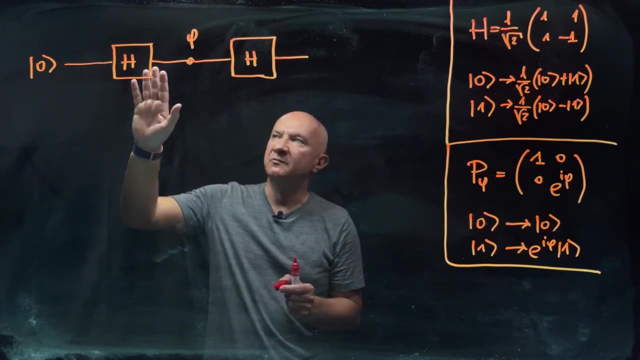 the phase gate. So let's step through the circuit and try to find out what are the probability amplitudes and the probabilities at the output. Of course, you know we can do it in a brute force way, So we can simply multiply matrices corresponding to the Hadamard, the phase and the 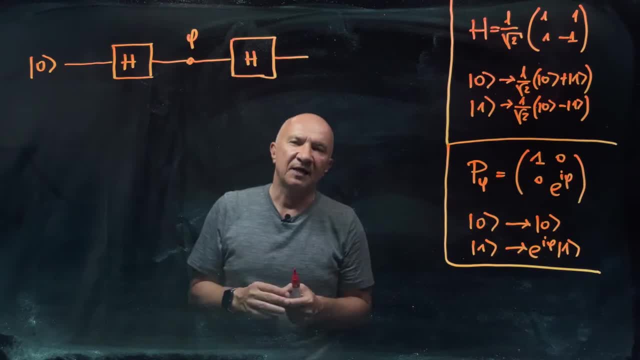 Hadamard. But that will be sometimes asking for too much because that would give us the input-output probability amplitudes. So we can simply multiply matrices corresponding to the Hadamard, the phase amplitudes for all kinds of different inputs. In this case we just fix the input at zero. We are 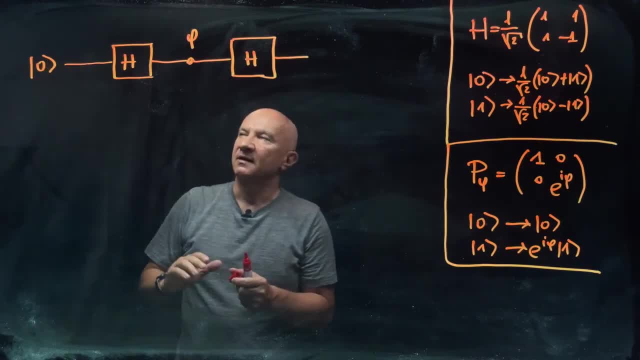 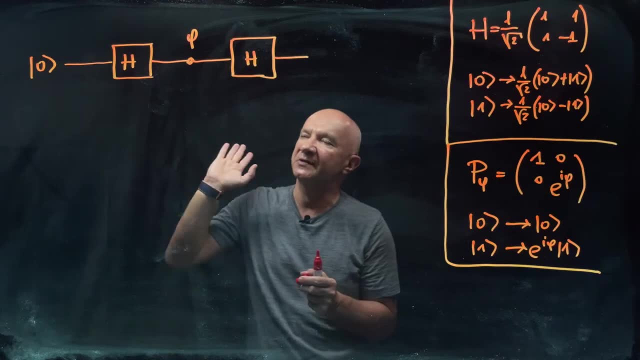 not interested in what will happen if the input is one. In this case, it's much easier and much more common in the community to step through the circuit, step through the network. Remember, sometimes I'll call this thing a network or sometimes it will be just a circuit You choose. 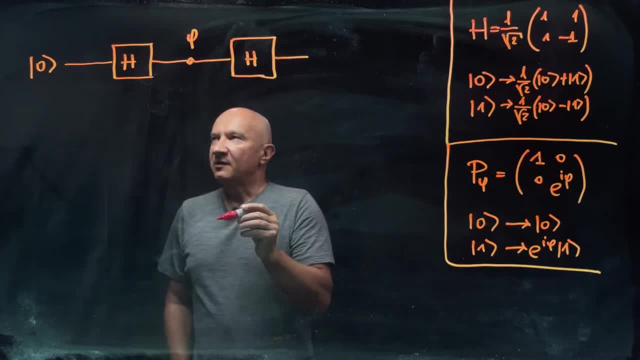 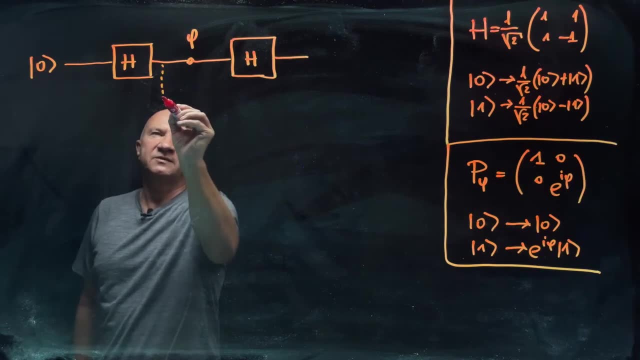 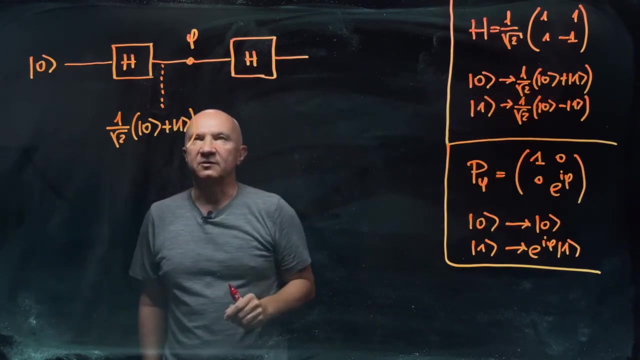 your word. So let's go. The first step, the Hadamard gate. so the state here at this point will be one over square root of two zero plus one right. So we use the definition of the Hadamard Zero. goes into this equally weighted superposition of zero and one. 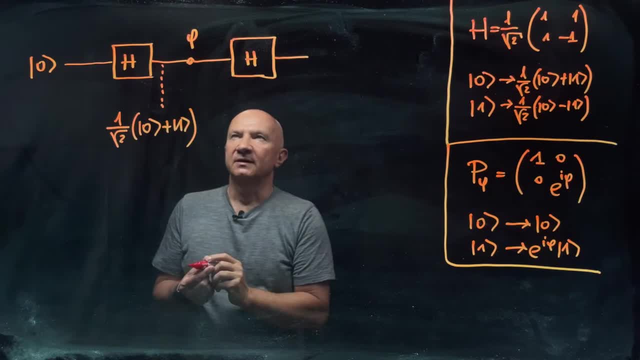 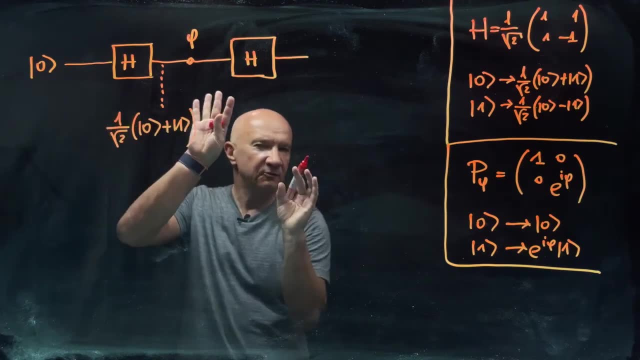 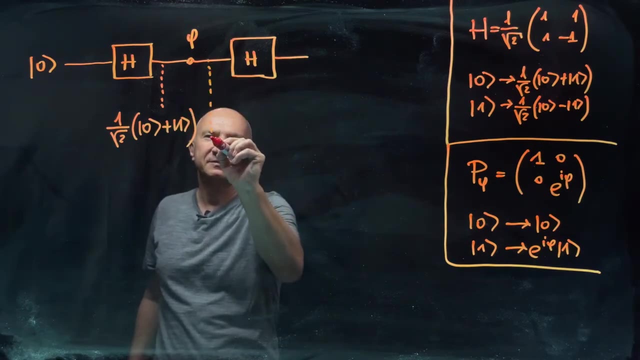 So that's the opening of quantum interference, Then the phase, very important element of any interference. It will control it all. It looks very innocuous, but pay attention, This is actually the most important gate here. So after the phase gate, the state will be 1 over square. 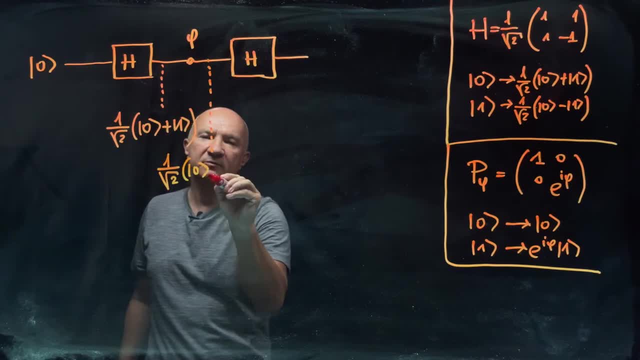 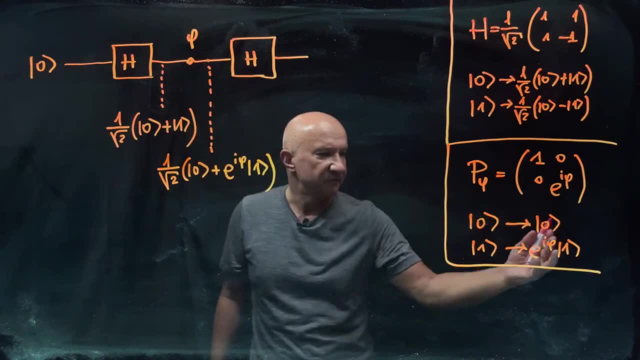 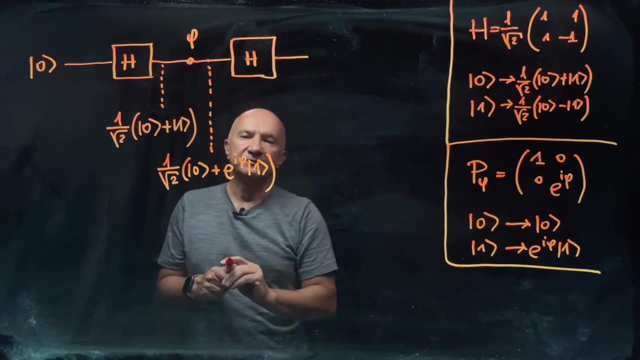 root of 2, 0 plus e i phi, 1.. So you see, I'm using this definition again: 0 survives, 1 gets the phase shift And now the harder mode again. So we are interested now what will be the state here. 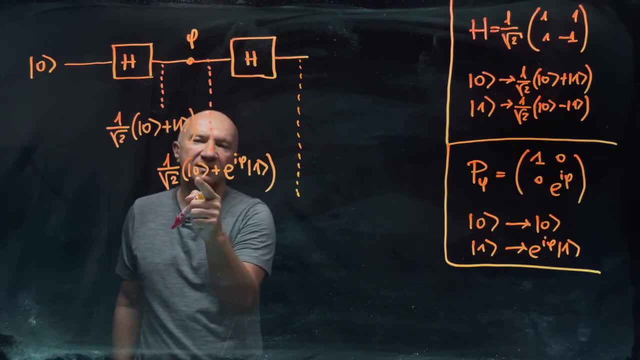 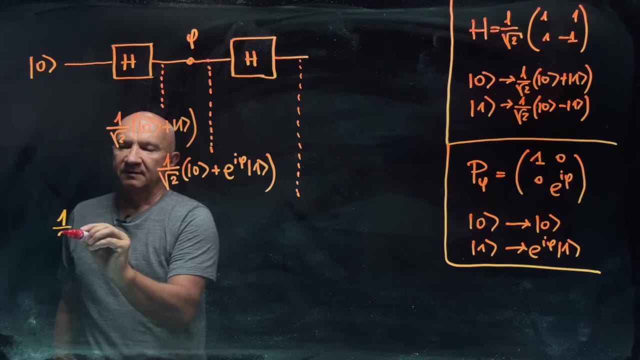 So, as you can see, the harder mode will take 0 into a superposition of 0 plus 1 and 1 into superposition of 0 minus 1.. And we also have 1 over square root factor here. So altogether we will have a state that will look like this: 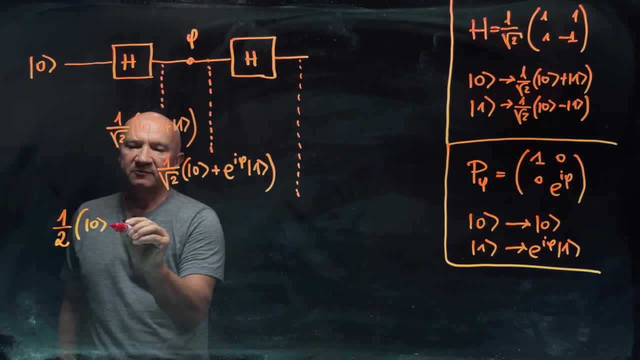 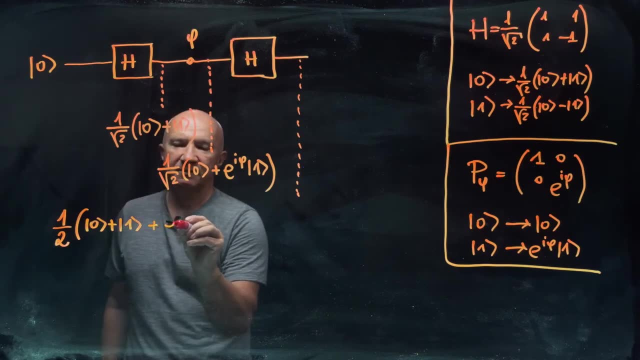 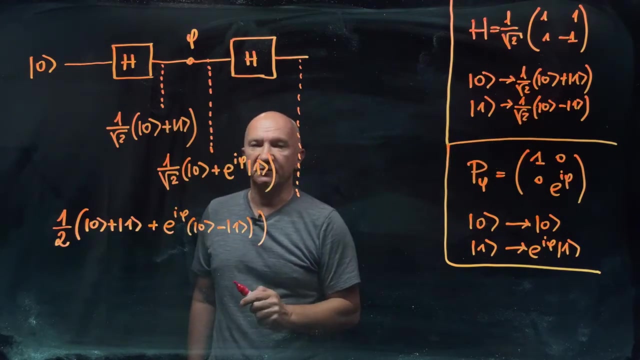 1 over 2, I have 0 plus 1.. That is from this part plus e i phi 0 minus 1, right, So this 1 is taken by the harder mode gate into a superposition: 0 minus 1.. 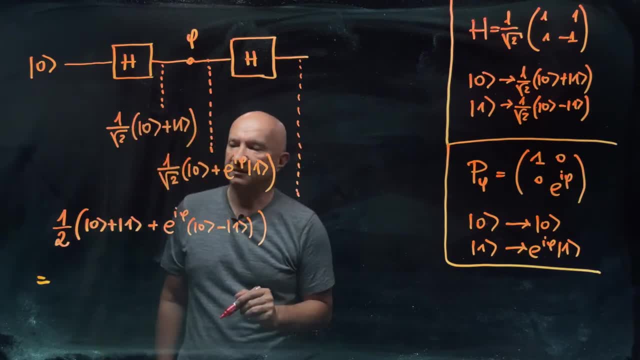 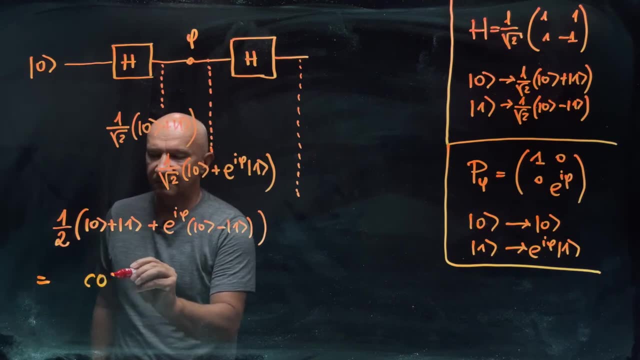 So this: then, if you just collect the terms and do all the necessary algebra, you will get you will get a state that will be 0, 1 over square root of 1.. So with this state we will get a state of infinity. 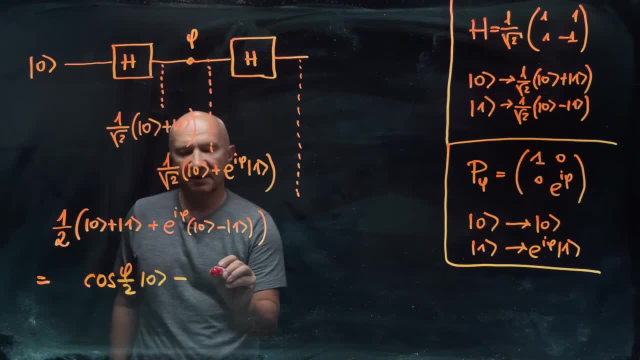 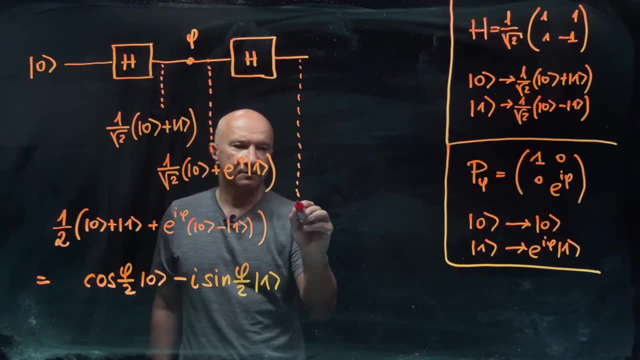 So that's 1 over square root of 1 plus 0.. So no more than that. If you want to get the answer, just take the negative. So 0 plus 1 is in fact the minus I sine phi over 2, 1.. 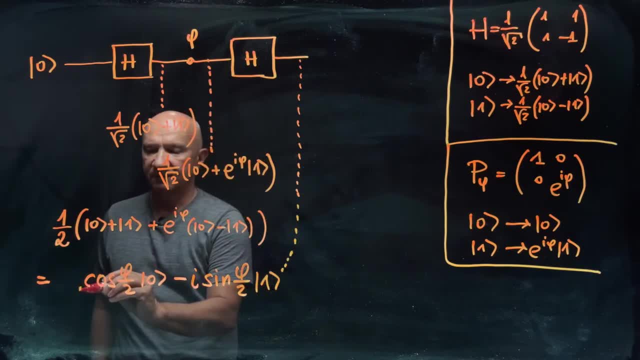 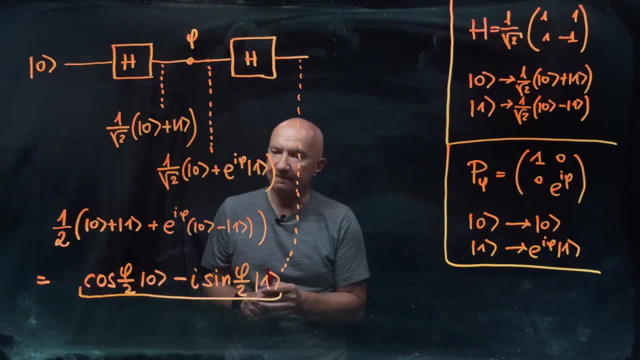 So this is the state that you get at the output. Now you look at this state at the output and you then can see that the probability of 1 over 2 is 0. And the next step is that the whole of the unit is going to be 0. 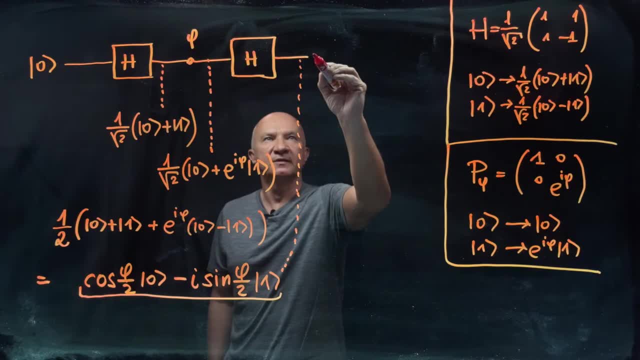 So the whole of the unit is going to be 0.. So 0 over 3 is 0.. All right, So the whole of the unit is going to be 0.. probabilities corresponding to finding zero or one are given by. so let me write those. 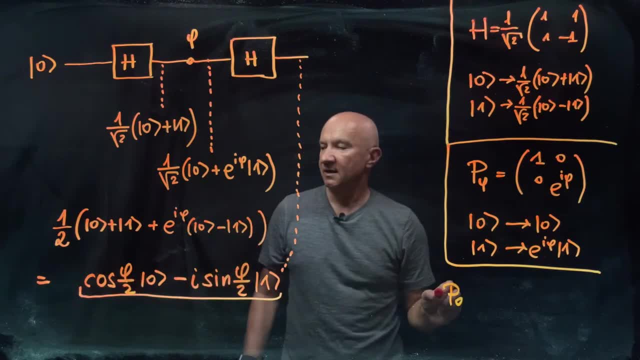 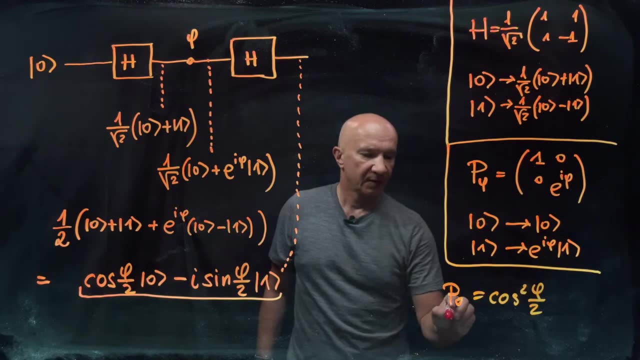 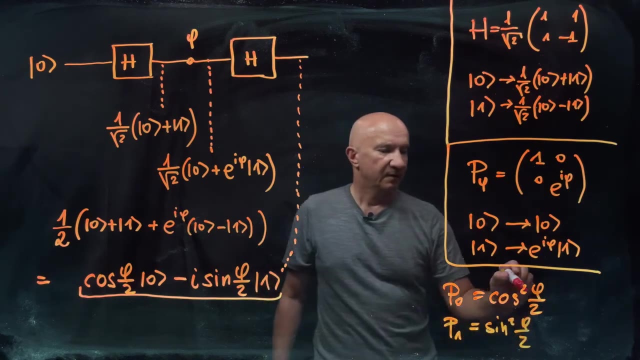 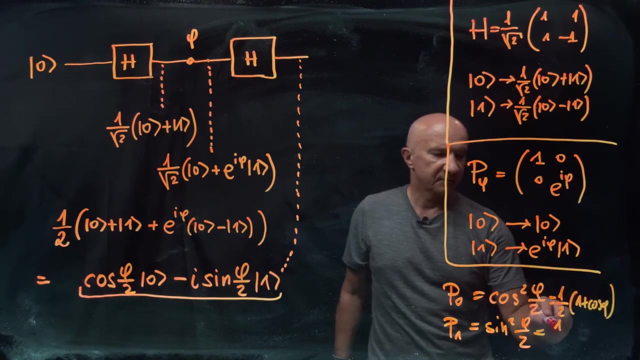 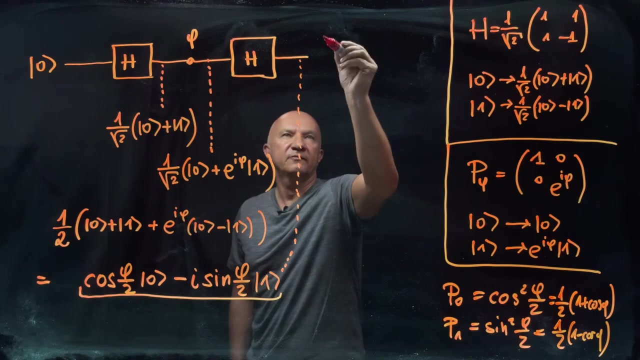 probabilities. probability that you'll find zero is cos squared phi over two, And probability that you find one is, of course, sine squared phi over two, which you can write as half one plus cos phi, and this is equal to half one minus cos phi. So if you're interested, 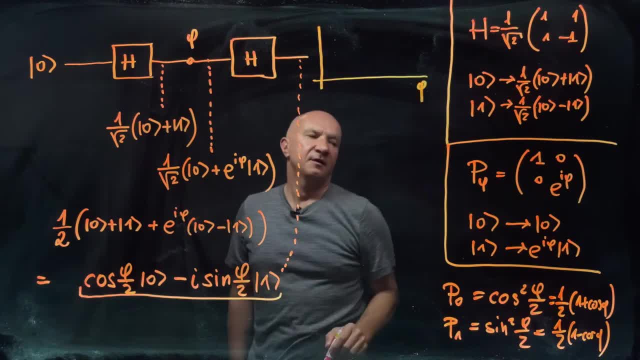 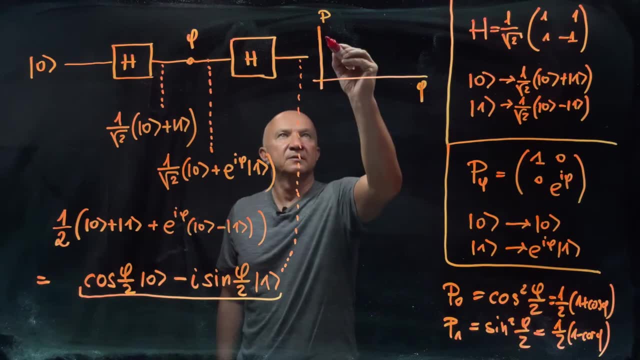 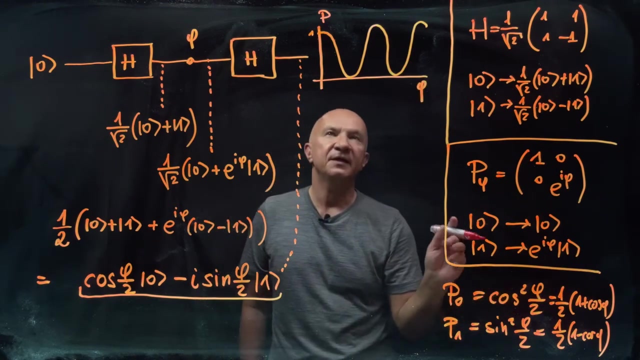 how this probability looks like as a function of phi. you can see that, for example, probability that you find zero oscillates. It starts from zero, from one, and it just oscillates, so that this expression here goes to zero when phi is equal pi, and then again.